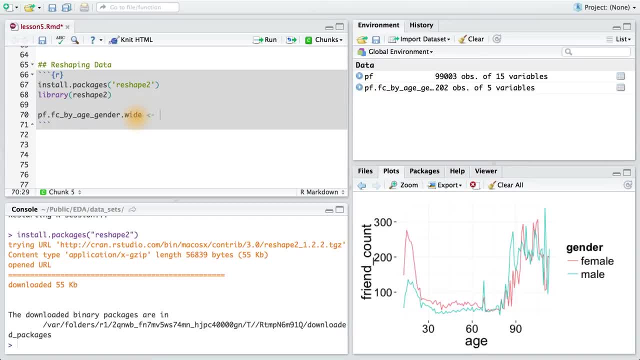 variable name for the data frame and just add wide to the end. Now we're going to make use of the dcast function which comes with the rshape2 package. The letter d is used since we want the result to be a data frame. If we wanted an. 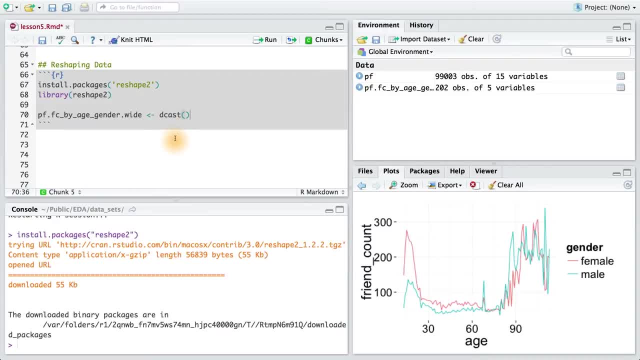 array or a matrix. we could use acast. We specify the data set we are going to change and then we put in a formula. So here's the data frame I want to modify, and then this is where I'll enter my formula. Now the first part of the 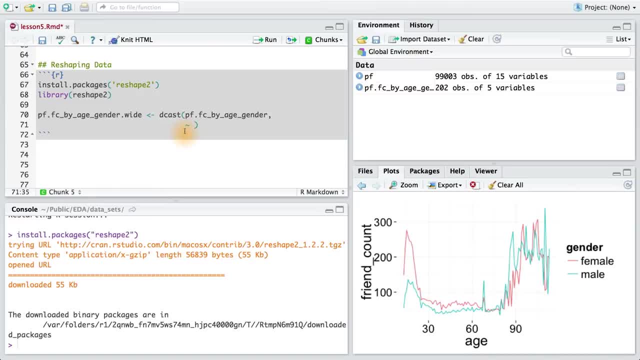 formula or the part to the left of the tilde sign will list the variables I want to keep with an addition sign in between them. Here I just want to keep age On the right side of the tilde. we use the gender variable since we want. 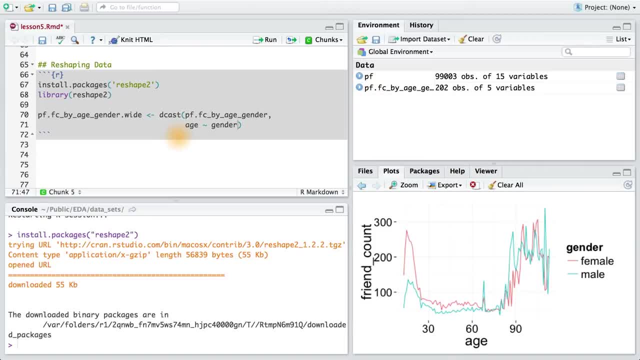 male and female users to have their own columns for median friend count in the data frame. And finally, we want to keep the gender variable, since we want female users to have their own columns for median friend count in the data frame. Finally, we set valuevar equal to median friend count, because valuevar 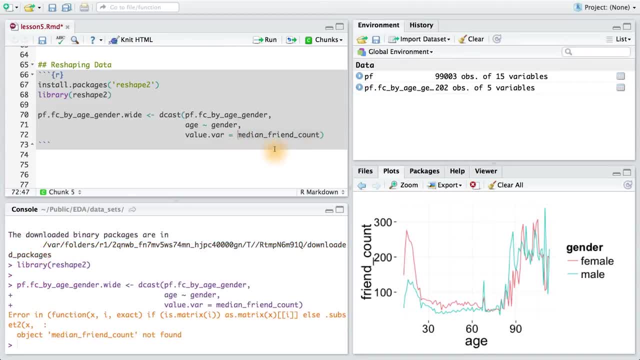 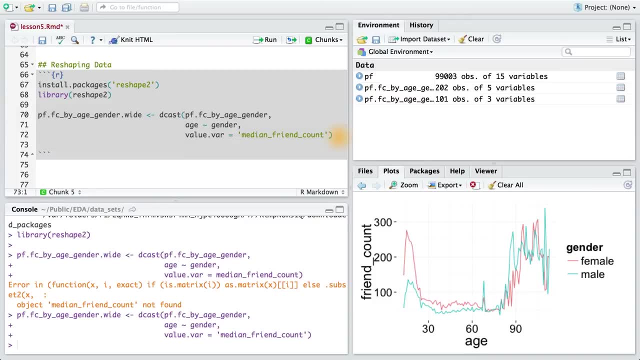 holds the key measurements of the values in our new data frame, And it looks like that I forgot quotes around this variable, so let me add that Now we should get a new data frame. Let's look at some of this data frame so that way.